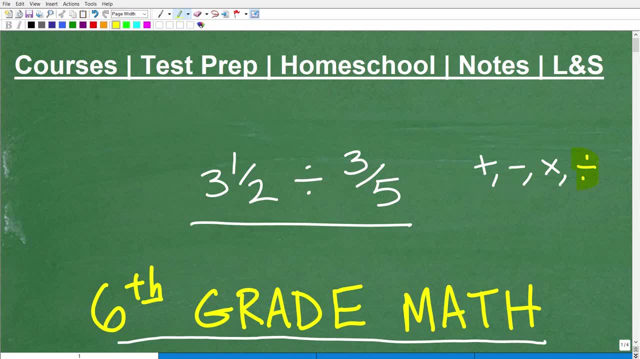 So 6th grade is probably where most students are really going to get into fractions big time. But if you're in high school, I can tell you right now there is a ton of students in high school, even college or just in general, that struggle with fractions. So if you need to review how to divide fractions, we'll stick around. I'm going to give you a quick crash course on this And I'm also going to give you some suggestions on how to add and subtract and multiply fractions as well. Matter of fact, we are going to be talking about how to multiply fractions. 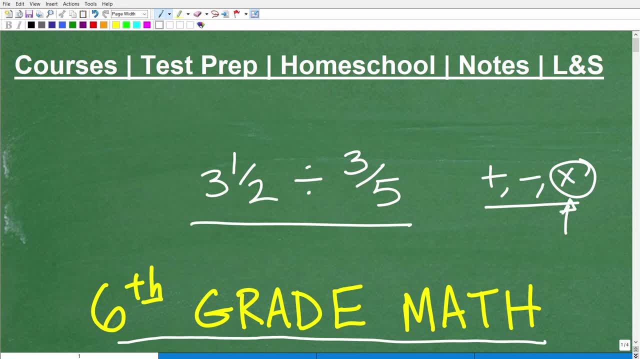 So stick around for a minute or two. if you've been struggling with how to divide fractions, This is not that difficult. But before we get going, let me quickly introduce myself. My name is John. I'm the founder of TC Math Academy. I'm also a middle and high school math teacher. I've been teaching math for decades And I'm telling you right now, if you're struggling in the mathematics, there's hope for you, And I put together what I like to believe is one of the best online math help programs there is. I'm going to leave a link to it in the description of this video. 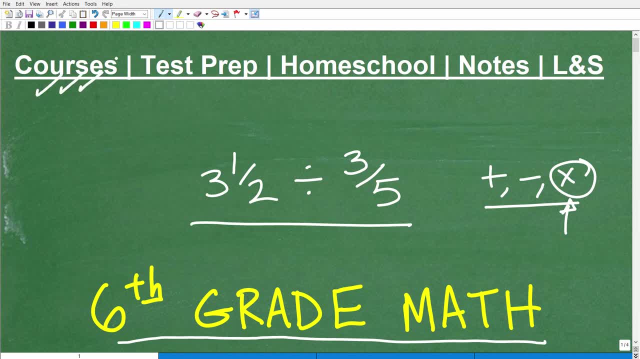 But if you're taking any level of math- middle school, high school or college- check out my math help program. I promise you you will like my instruction- Very robust programs to help you out in your respective math courses. Also, if you're preparing for any sort of test, something with a math section, like the GED, ASVAB, SAT, teacher certification exam- I have a ton of test prep courses that can help you out. If you homeschool, I have an excellent homeschool program. By the way, if you need some comprehensive math notes, I'm going to leave links to my 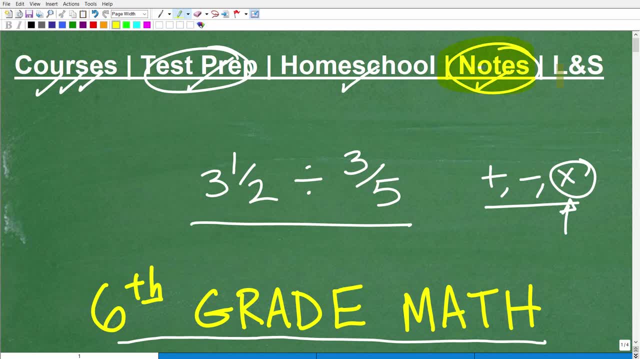 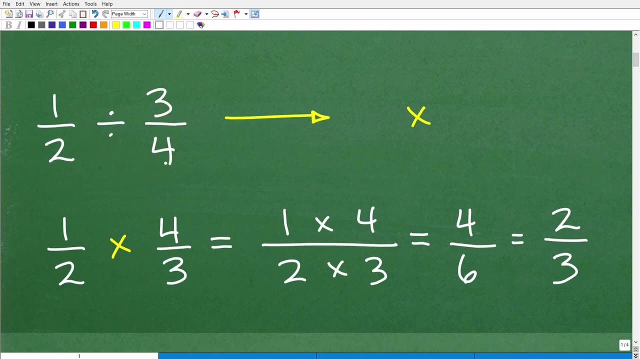 notes in the description of this video, And if this video helps you out, don't forget to like and subscribe, as that definitely helps me out. And with all that being said, let's get into how to divide fractions. Well, here's the thing, When we're dividing fractions- and so let's take an example like this one: half divided by three, fourths- This is the operation that we want to do. We want to do division. However, we really don't divide fractions per se. What we do is we take a 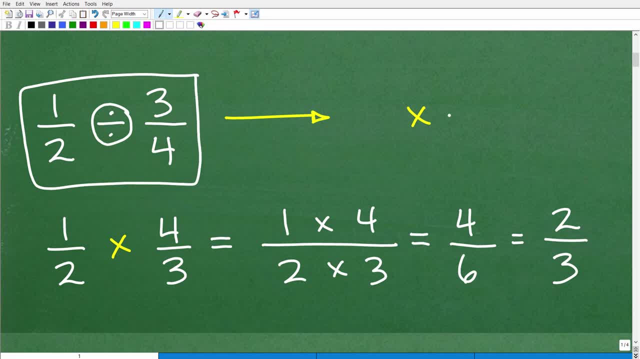 problem like this, a division problem, and we're going to rewrite it into a new problem involving multiplication. Okay, so we're going to take all of our division problems and turn them into multiplication problems, And that will be effectively how we divide fractions. So let's go ahead and take a look at this problem: One half divided by three, fourths. I want to turn this into a new problem that involves multiplication. So what do we do? Well, this is how it works. Okay, so what we do is we take a 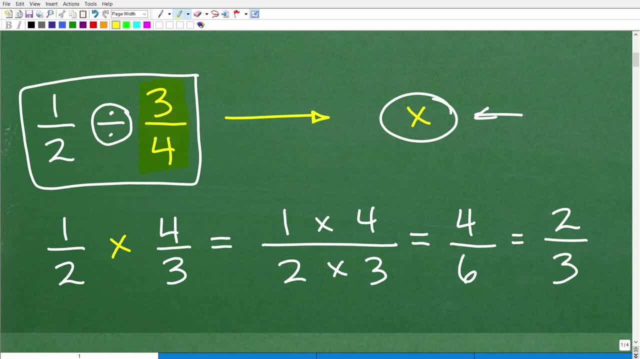 we have to do is go to the fraction to the right of the division operator. So this is the division operator right here. This is the fraction to the right of it. This is the fraction to the left of it. We're always going to focus in on the fraction to the right of that division symbol. Okay, so 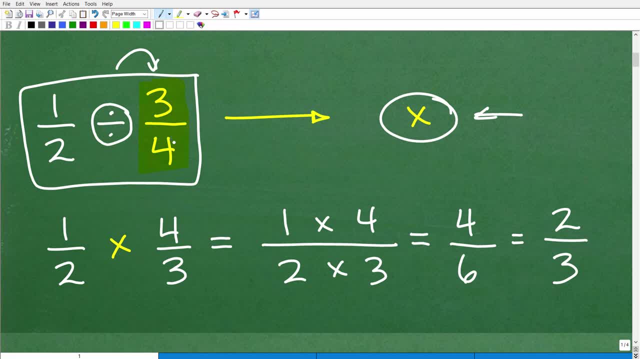 there. it is right there, and we're looking at the fraction three-fourths. So what we're going to do is we're going to take this fraction here and we're going to flip it upside down. That's called the reciprocal. So instead of three over four, we're going to write this as four over three. 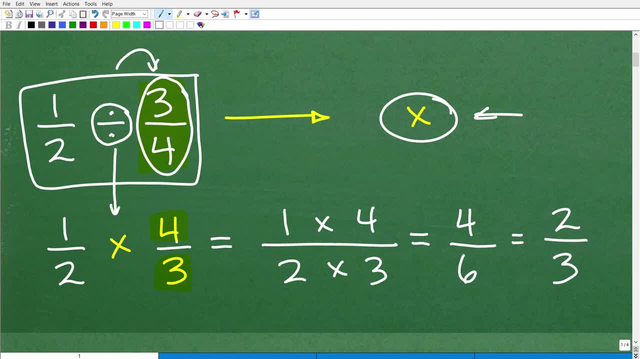 Okay, and when we do this, we're going to change this division symbol into a multiplication symbol. Okay, so we're going to go from a division problem into a multiplication problem by flipping the fraction to the right of that division symbol. Okay, so hopefully that's clear enough. Let me 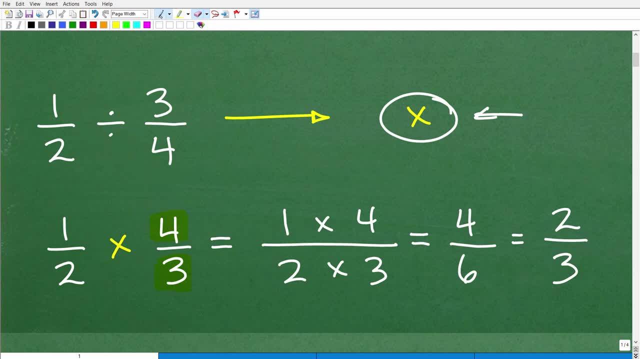 erase all of this and we can kind of see here: All right, so one-half divided by three-fourths. Well, I'm not going to do division, I'm going to do multiplication, and so I'm going to write this as one-half times. but I'm not going to write. 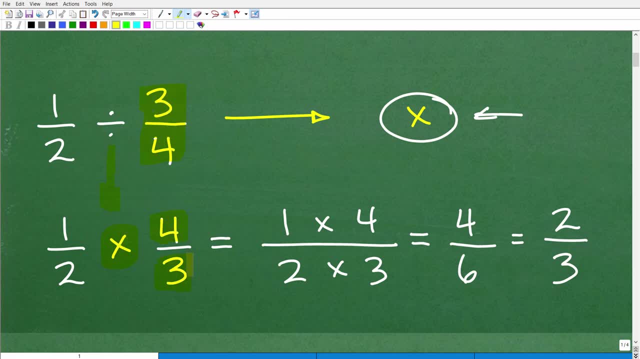 three-fourths. I'm going to flip this fraction as four-thirds. All right, so now we have to know how to multiply fractions, and this is super, super easy. The way we multiply fractions is we multiply the respective numerators and denominators. So the numerators are the top numbers of the 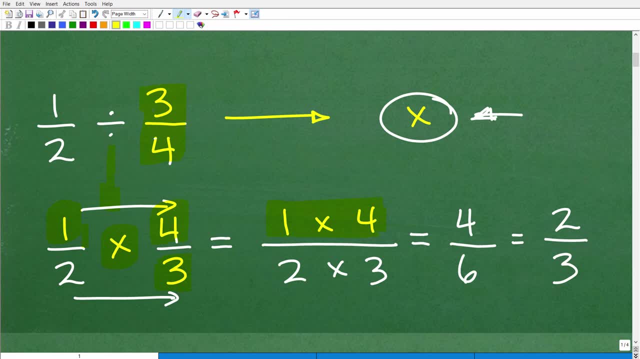 here We're going to multiply one times four. Okay, those are the numerators. and then we're going to multiply the respective denominators. That's two times three. So one times four, of course, is four, and two times three is six. So we have the answer four-six, but we can reduce that. 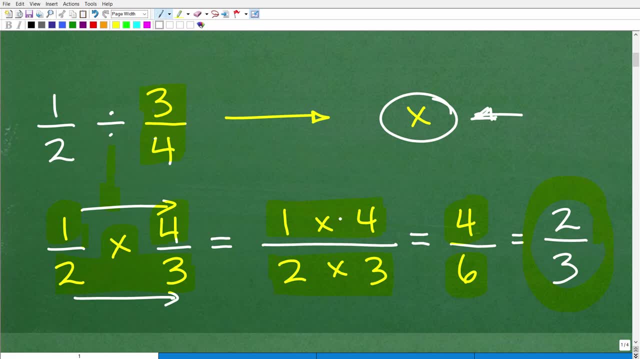 as two-thirds, and if some of you are really up to speed on your fractions, you could say: well, here this two can go into that four-two. so that just gives us the fraction two-thirds. but you always want to reduce your. 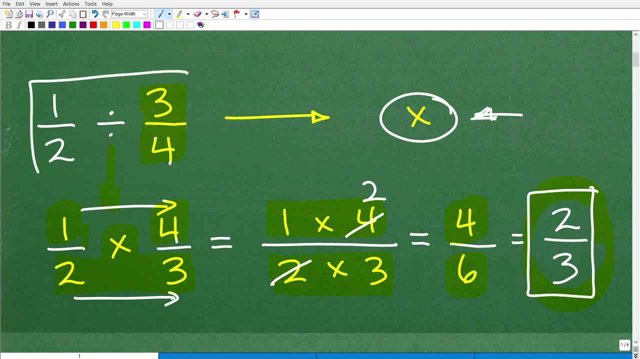 final answers. But anyways, let's just review here. Here we had a division problem of fractions: One-half divided by three-fourths. We turn this into multiplication. by finding the reciprocal of the fraction to the right, We multiply the respective numerators and denominators. This 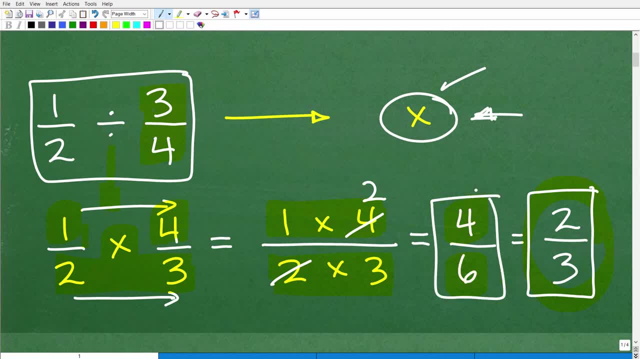 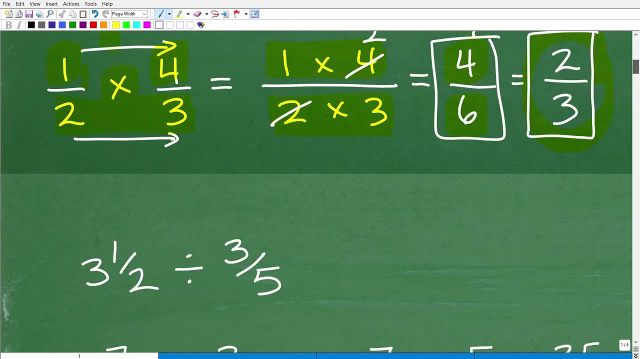 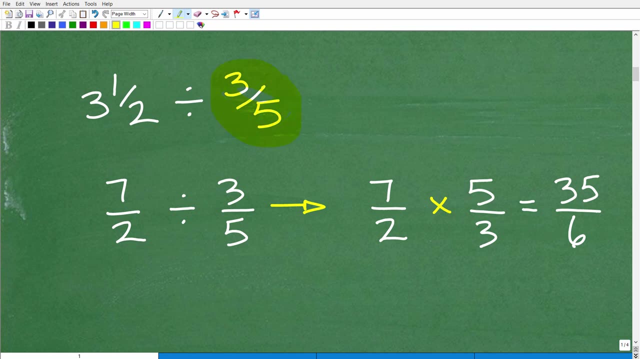 is how we multiply fractions. We got our answer and then we reduced our final answer, and there you go. All right, so that's all you need to do. but let's take a look at a couple other variations when we're dealing with division of fractions. So when you have a fraction like this, let's just 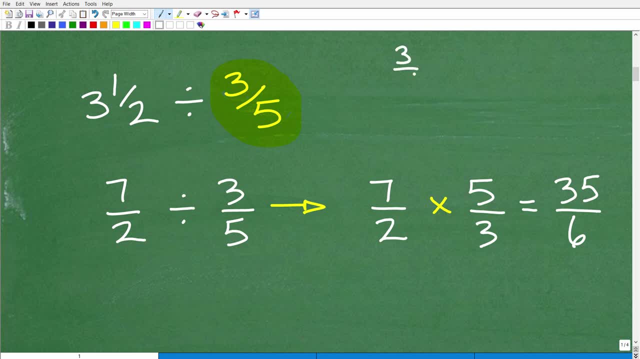 review some basic terminology like three-fifths. This is called a proper fraction. okay, So you can see here it's not like this fraction. This is what we call a mixed number. So a proper fraction is where the numerator is greater than the denominator. right, So you can see the denominator. 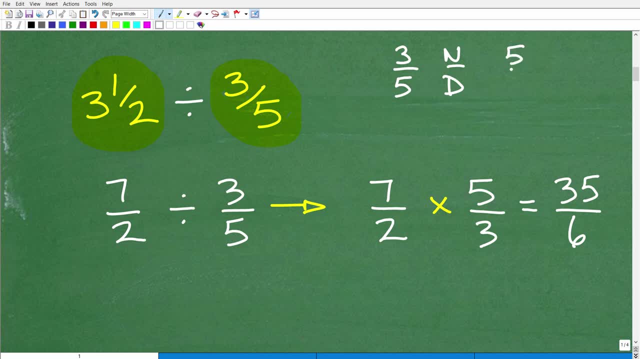 is bigger. Now, an improper fraction is where the numerator is larger than the denominator, so something like five-thirds. okay, So this is an improper fraction, this is a proper fraction and this is a mixed number. So we're going to have to deal. 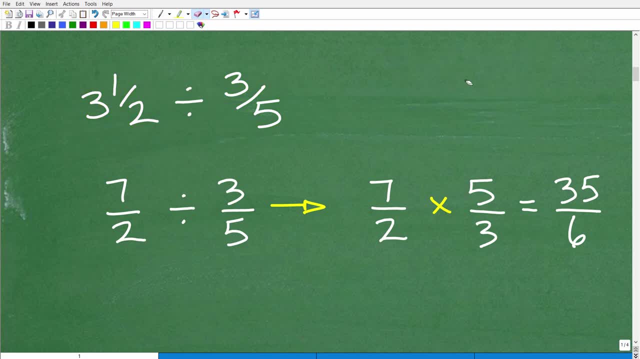 with all these different types of forms of fractions, but the procedure stays the same. So let's go ahead and talk about how we're going to do this problem. So we have three and one-half divided by three-fifths. So, again, what we're going to do is we're going to change this division. 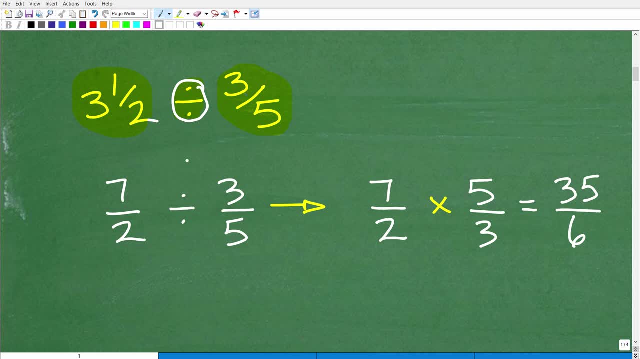 into a multiplication problem, but we can't do this just quite yet, So what we're going to do is focus in on writing any mixed number fractions as improper fractions. okay, So we're going to rewrite three and one-half as seven-halves, So remember the way we do that. let me just write. 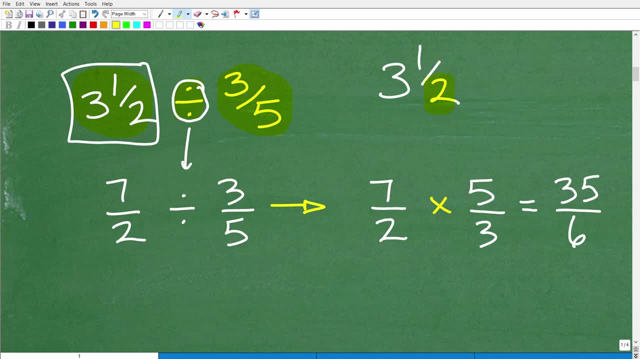 this really big over here. three and one-half. so you're going to say, oh, two times three is six. six plus one is seven. so three and one-half is the same thing as seven-halves. okay, So it's just a quick review: how to change a mixed number into a 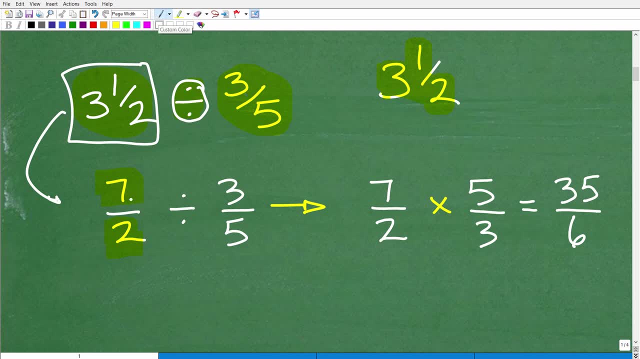 improper fraction. okay, So now we have, instead of three and one-half divided by three-fifths, we have seven-halves divided by three-fifths, and now we can go ahead and go to our procedure. So here we have that division symbol. We're going to go ahead and flip this fraction to the right. 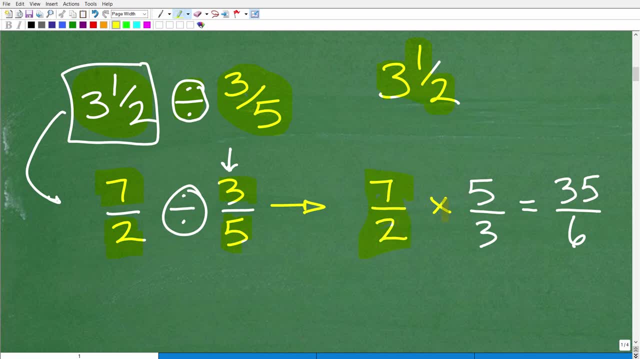 So this is going to be seven-halves times, okay, not. we're going to change that to multiplication, and then we're going to flip this upside down: Instead of three-fifths, we're going to have five-thirds, and now we can go ahead and just go. 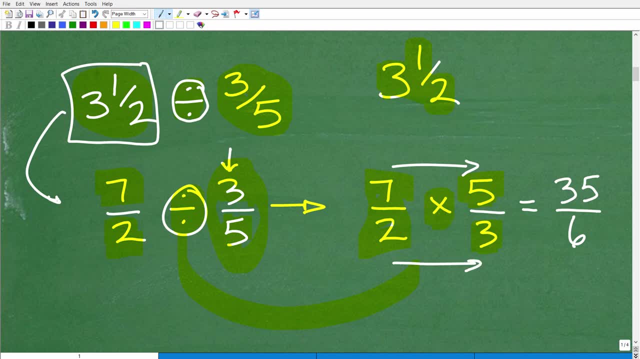 ahead and multiply the respective numerators and denominators. So seven times five is thirty-five, and two times three is six, and there you go We are done. Now. at this point, what we're dealing with here is an improper fraction. okay, This is an improper fraction. A lot of you are going to 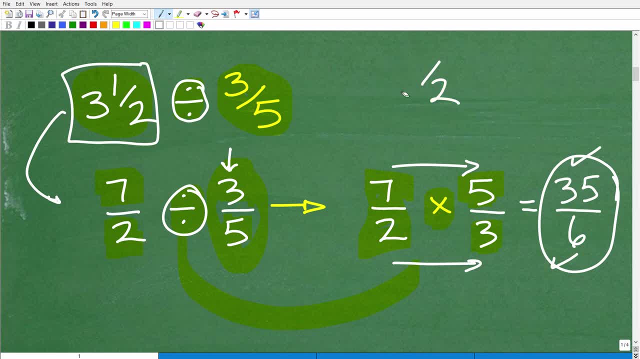 want to go. oh, should I just take this? No, not three. Let me write this right here: Should I take my improper fractions and turn them into mixed numbers, ie should you take six and divide it into thirty-five and then do all this? 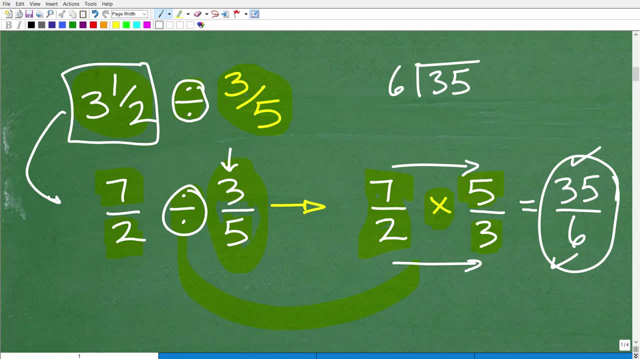 remainder and stuff. Don't do that. okay. You need to know how to do that, but don't do this as a general rule. okay. What you need to do is leave your final answers reduced. Just leave things like this. I've seen so many students have the correct answer in terms of an improper. 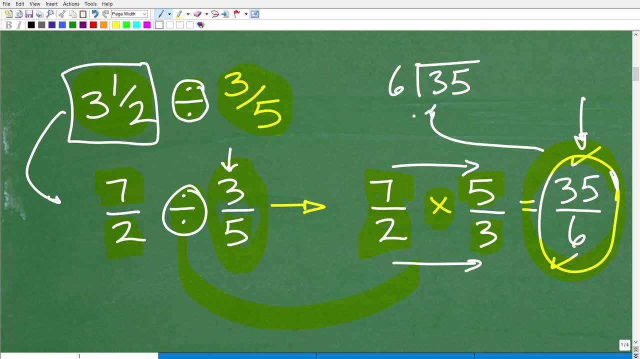 fraction, but they go, try to take their improper fraction and turn it back into a mixed number and they make a mistake and then they turn in the wrong answer. So do not do that. Okay, so let's go ahead and continue to practice with mixed numbers, So we'll finish up with this. 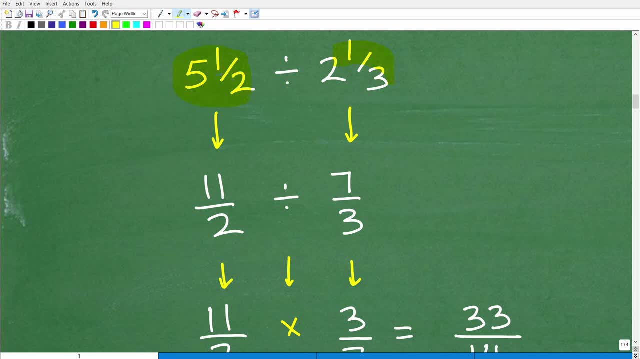 problem. So here we have five and one-half divided by two and one-thirds. Again, you can't do anything until you get all these mixed numbers if you have them written as improper fractions. So five and one-half is going to be two times five. 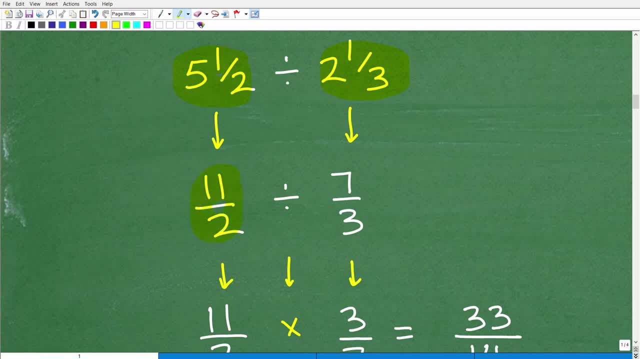 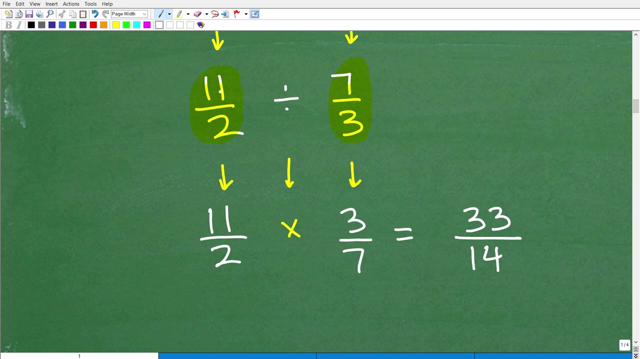 Five is ten plus one is eleven-halves, divided by two times three is six plus one is seven-thirds. Okay, so the first step I'm going to do is just rewrite this problem with improper fractions. So now I have a division of improper fractions: eleven-halves, eleven over two, divided by: 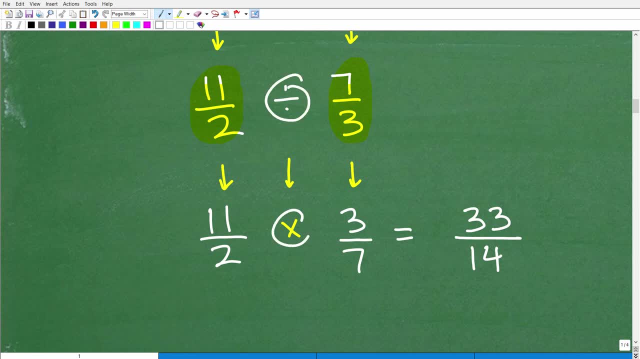 seven-thirds. So I'm going to change this division into multiplication by flipping this fraction to the right, So that will be, instead of seven-thirds, that'll be thirty-five, So that'll be three-sevenths. And now I can go ahead and multiply across our respective numerators. 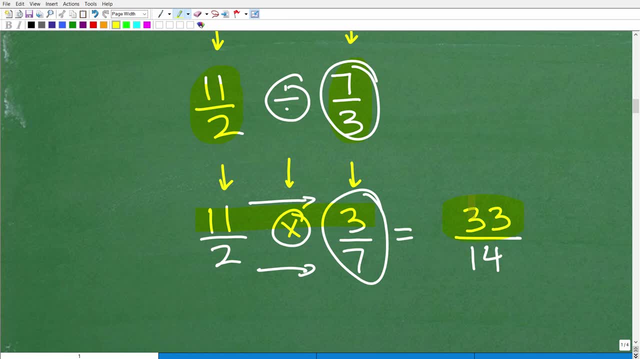 Eleven times three is thirty-three, and then two times seven is, of course, fourteen. And you do look to say, hey, can I reduce this? Well, this cannot be reduced, so then you would be good to go, All right. so hopefully we took a look at enough variation of how to divide fractions with mixed 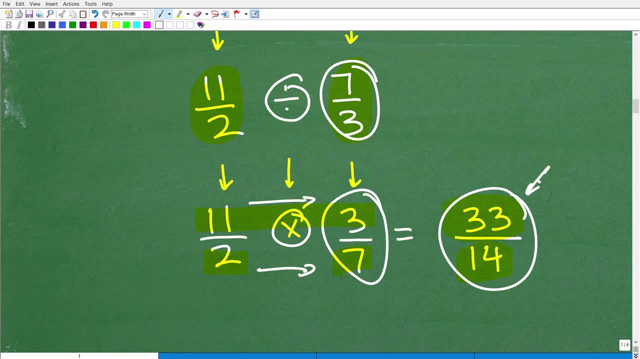 numbers and improper fractions, et cetera. Notice, one thing that I didn't do here is I didn't have any positive or negative numbers. In other words, we're not doing like negative three-halves divided by positive one-fourth, for example. That's another kind of level. 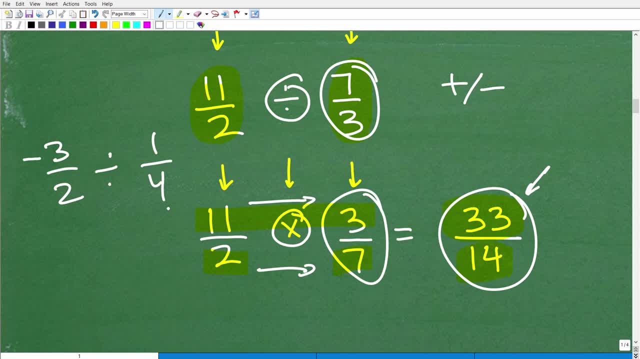 of mathematics and you still learn this at the middle school kind of level. But I kind of wanted to just focus in on the basic operation of dividing fractions. Okay, you want to get that down. and then, of course, you need to know your rules for positive and negative. 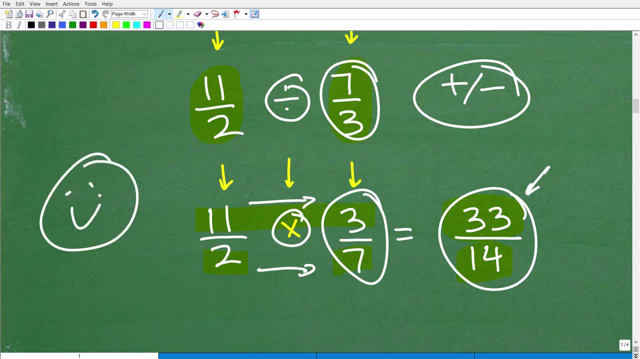 numbers. Have you done enough already? Well, I must go ahead and give you a nice, lovely, happy face, an A plus plus a 100 percent and a few stars, so you can feel extra special today. But if you 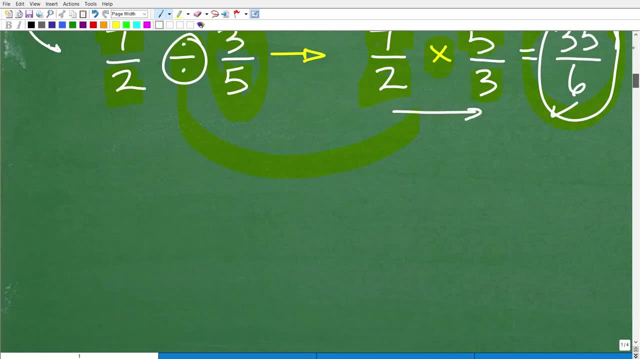 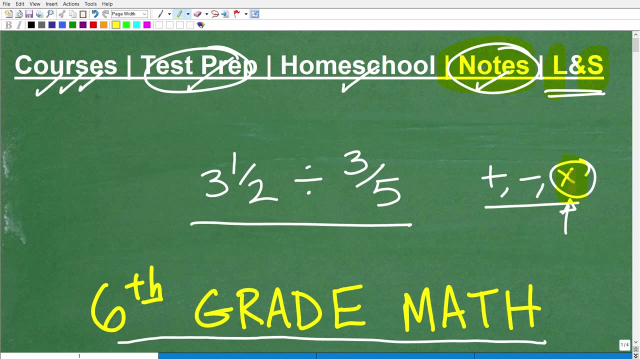 need additional help with fractions, positive and negative numbers, et cetera, et cetera. I'm going to go ahead and give you some suggestions, because, of course, we talked about how to multiply fractions and divide fractions, but where students really struggle with is how. 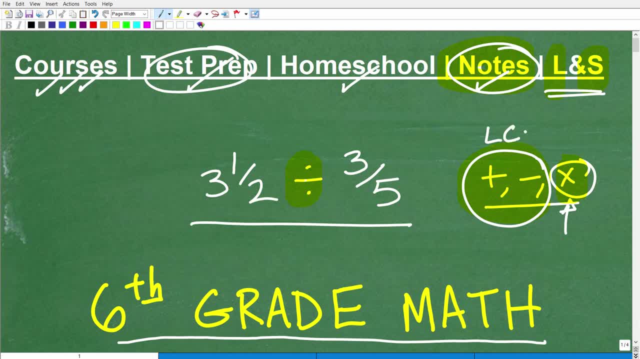 to add and subtract fractions, because this is where you generally have to deal with all that LCD stuff et cetera. So a couple of suggestions if you still need help with fractions as an overall topic One: I have a ton of videos on my YouTube channels that 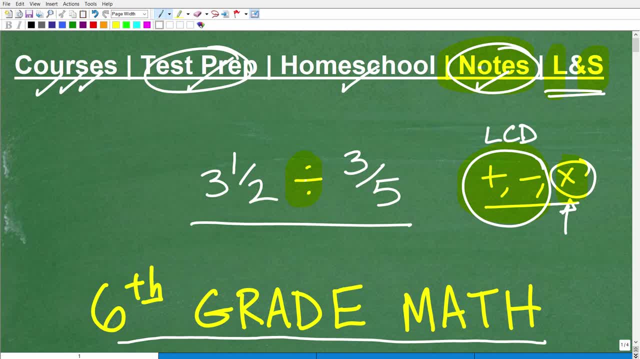 can help you out on fractions, adding, subtracting, how to reduce fractions, how to convert fractions to decimals and vice versa. Or you may want to check out one of my courses, like my pre-algebra course or my math foundations course. I really get into all this and much, much more Of.